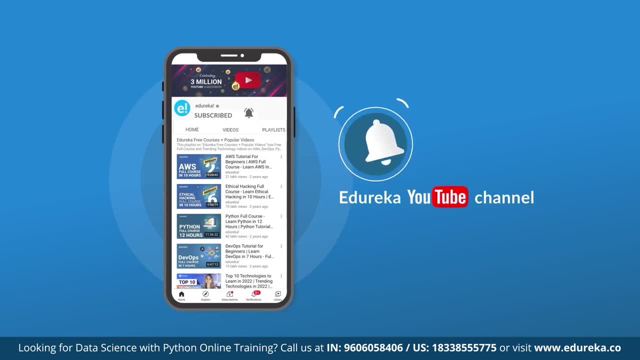 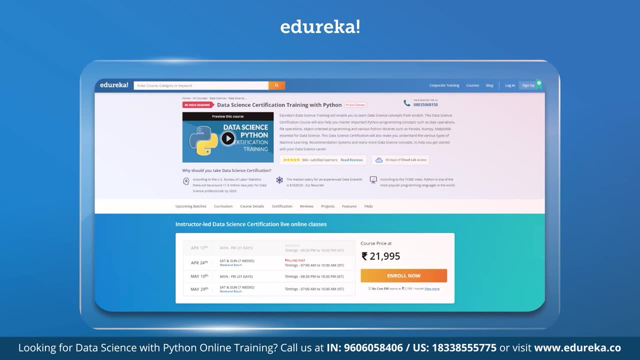 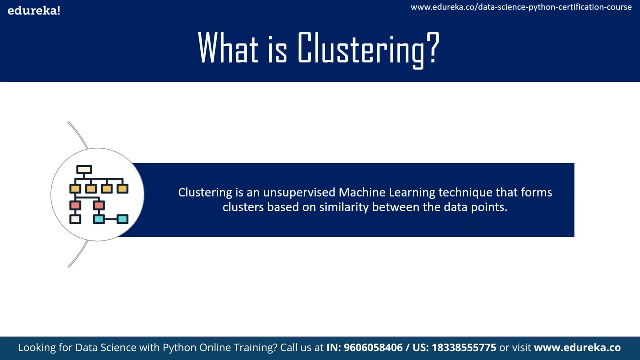 sure you subscribe to Edureka's YouTube channel and hit the bell icon to never miss an update. also, if you are interested in online training certification, do check out the link given in the description. so now, moving on further, let's understand what is clustering. so clustering is an. 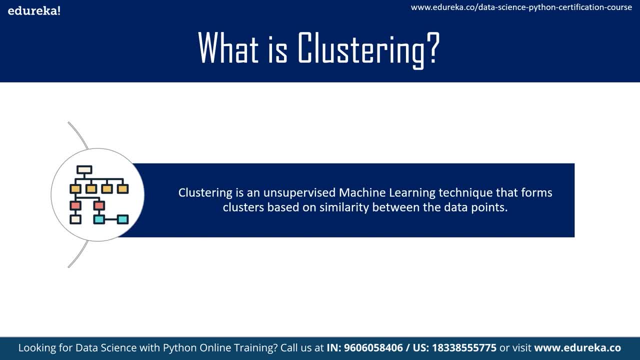 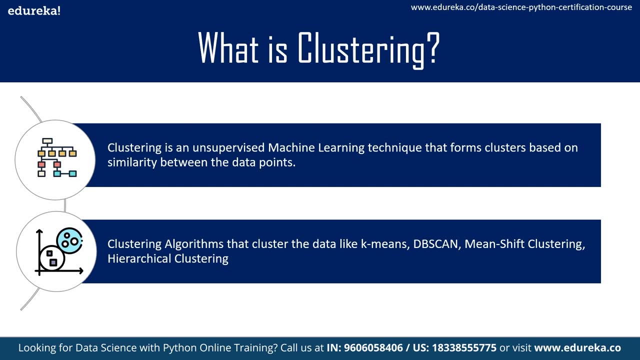 unsupervised machine learning technique which forms clusters, which is based on some similarity between the data points. okay, let me make things very clear and very simple for you all by explaining a few examples also of clustering. so there are various clustering algorithms that cluster the data, like k-means, db-scan. we've also got mean shift clustering and there's also Gaussian. 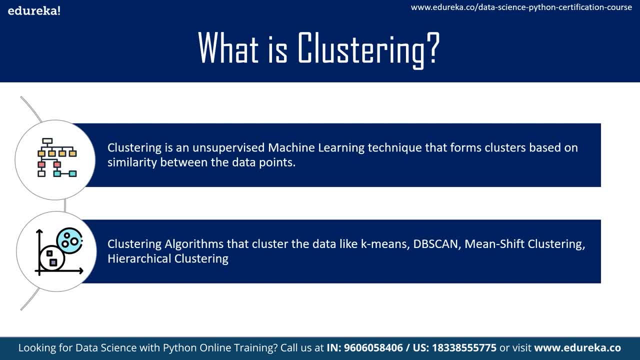 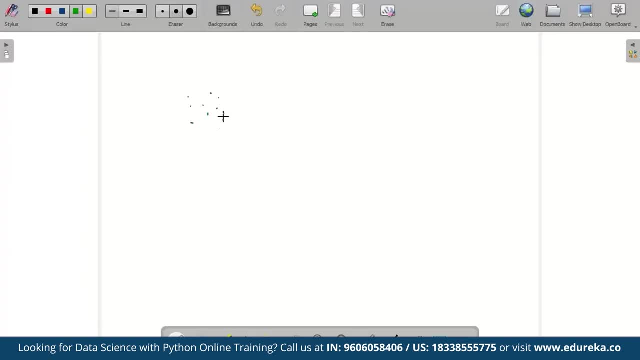 mixture models and hierarchical clustering. so the way the data points are clustered, they differ from each algorithm and today our focus is hierarchical clustering. so now let us understand what really is clustering. suppose I have some data points and I make a cluster of these data points and name it as X. 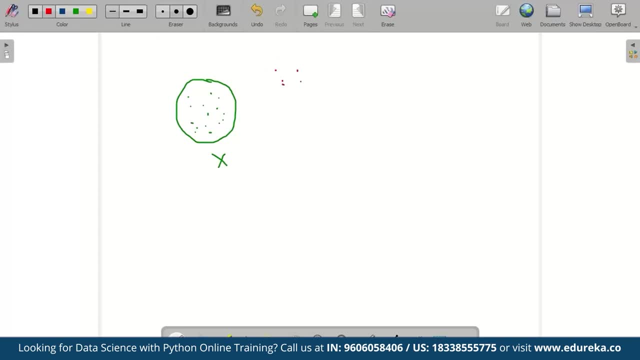 all right, and I have got another data point, set of data points- this is from my data and I cluster it in one another cluster which is named as five. now understand one thing very clearly: that the data points in this cluster are similar, based on certain similarities. so I can say that this data point and 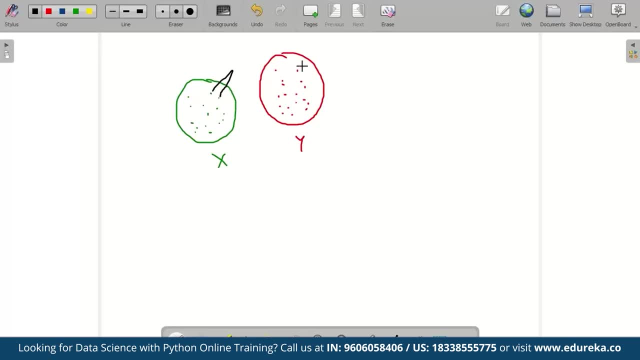 this data point they have some similarity. similarly, in cluster Y, this data point and this data point they share some similarity. but another difference is here is that the data point here in cluster X and here in cluster Y they are different based on certain dissimilarity. right, so we form cluster based on certain similarity and 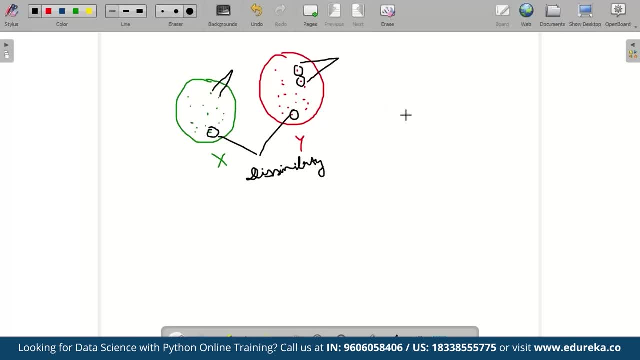 based on certain dissimilarity. so now let us understand the concept of hierarchical clustering. suppose I've got these clusters and I want to plot them. I have this X, then I have got this Y, and suppose there's another cluster called Z. now I see that cluster X and Y are somehow linked, so I cluster them into one like this: if I just cluster the 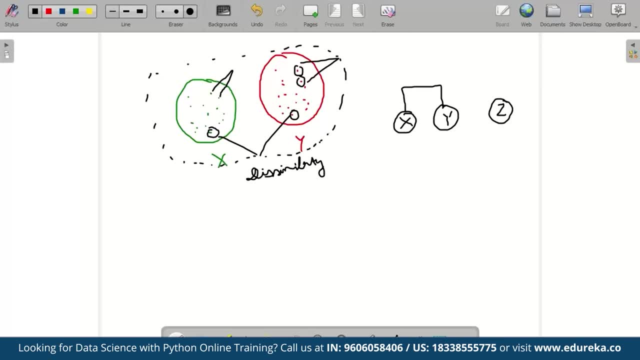 entire X and Y into one single cluster. then this is how I would represent it, and then Z would be linked in a different manner with X and Y- suppose this is again a Z cluster here- and then again I would form one another separate big cluster which will cluster all these. 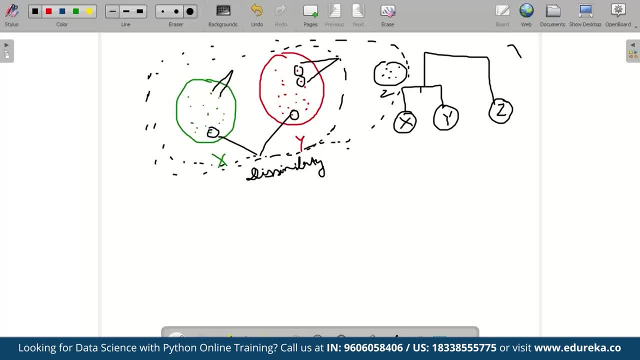 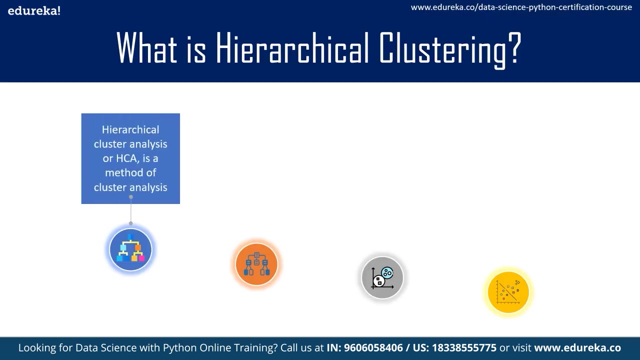 clusters right. so this then I have this- levels of clustering. this is known as hierarchical clustering, and the way the hierarchical clustering takes place is via agglomerative and divisive approach. so we will be discussing this agglomerative and divisive hierarchical clustering in our upcoming slides. so for now, let's just understand what is hierarchical clustering. so hierarchical clustering. 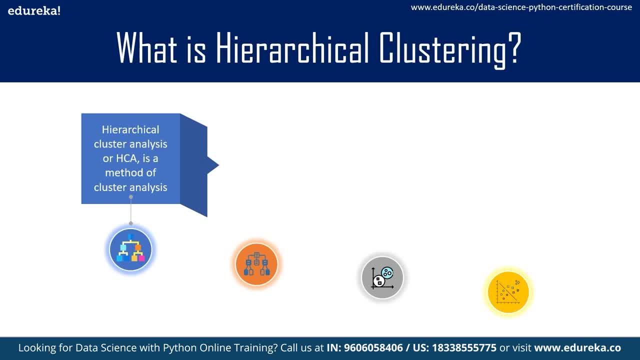 it is also known as HCA, or hierarchical cluster analysis, and this is a method of cluster analysis, as we have seen. so what happens here is that this clustering allows us to build the tree structure from data similarities, like we have built X and Y and we have created trees. 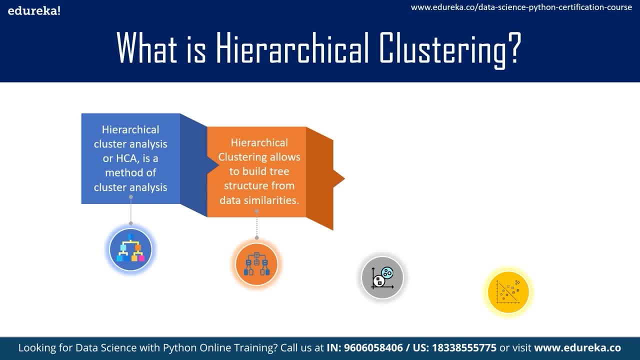 and these trees are actually called known as dendograms. so the way you represent a hierarchical cluster or hierarchical clustering, is through dendograms. so we actually drew a dendogram. okay, so this is how the clustering has been formed and this is how the clusters are being made. 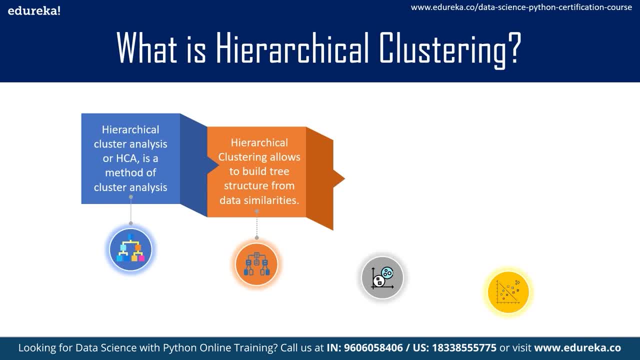 and this is how the relationship among the clusters has been shown by a dendogram. so based on these things now we will go on further to understanding what is agglomerative clustering. so when this hierarchical clustering follows a bottom-up approach, this is called agglomerative. 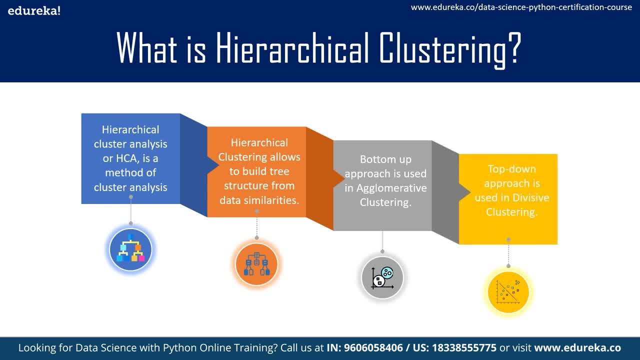 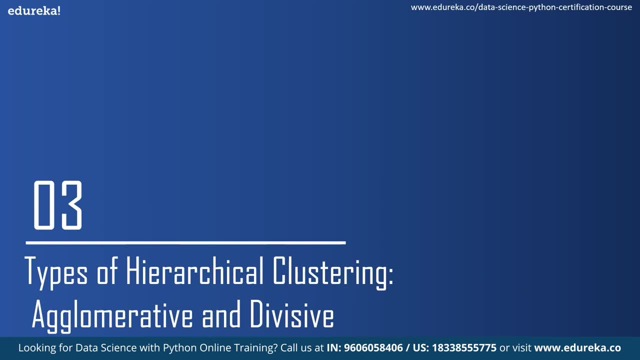 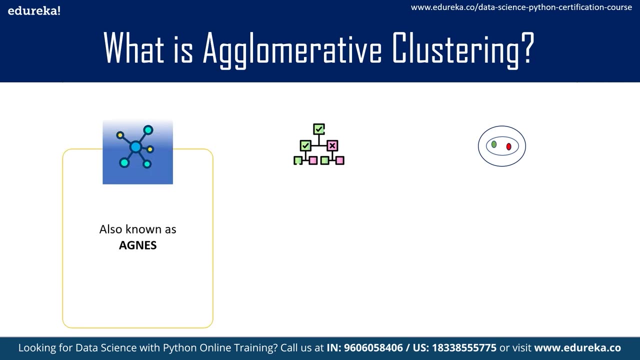 clustering and when this is following up a top-down approach. this is used in divisive clustering. so now let us understand what is agglomerative clustering, so the types of hierarchical clustering. so now, moving on further, what is agglomerative clustering? so agglomerative hierarchical clustering. 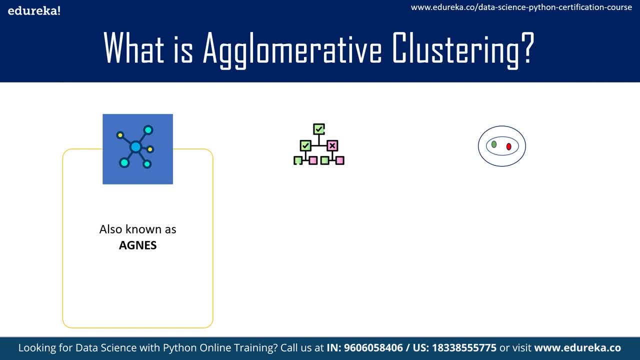 this is also known as agnes, which means agglomerative nesting, hierarchical clustering, and it follows a bottom-up approach, which means that clustering or clusters, they are formed from the bottom and are again clustered till a complete single cluster is formed, and what happens then is that the clustering 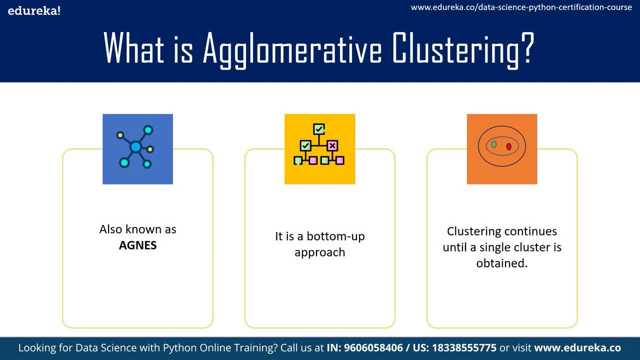 continues until we obtain a single cluster, and we will see how we obtain a single cluster and we also present it. so individual data points are clustered based on similarity and we go on clustering until there is only one single cluster on there. so let us just plot this agglomerative clustering and 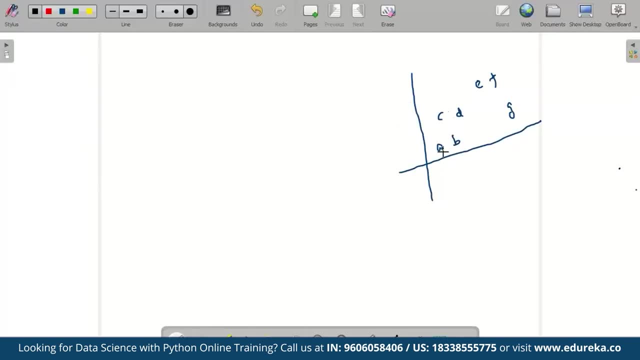 make things really simple for us. now suppose I have got these data points scattered here- a to g- and these data points have to be clustered. so another important thing is that now we will form clusters. so how clusters are formed, so we can see that, based on some similarity, like because of the 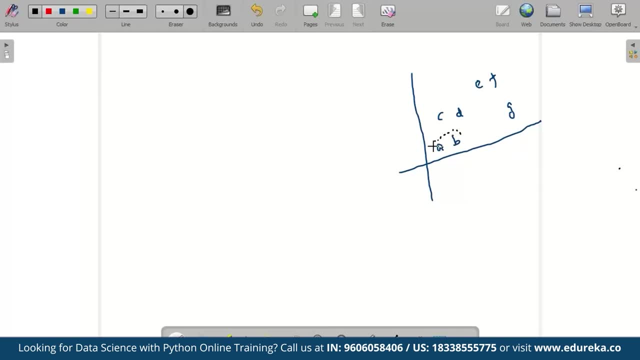 distance, nearby distance. a and b can be grouped together in a single cluster. so I am just doing that. c and d, I form another cluster because they are near, so I just club them. and again, I would just club e and f based on their distance, and g is separate, so I will just form a separate cluster. now what happens in? 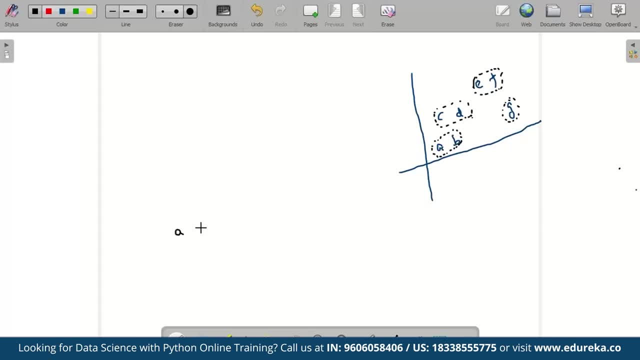 agglomerative clustering is that I have to plot all these data points like a, b, c, right d, e, f and g. so these are separate clusters. the clustering starts from the bottom and each data point is treated as a single cluster, which you will also understand with the help of an example further. but now for 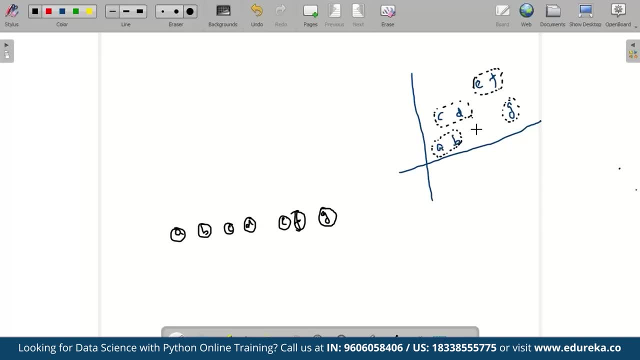 simplicity. let's take a, b, c, d, so then what happens is that, since a and b are grouped as one cluster, so this is how I just group them, all right, and c and d is grouped as one cluster. this is how I group them. e and f are grouped in one single cluster. this is how I group them. now remains 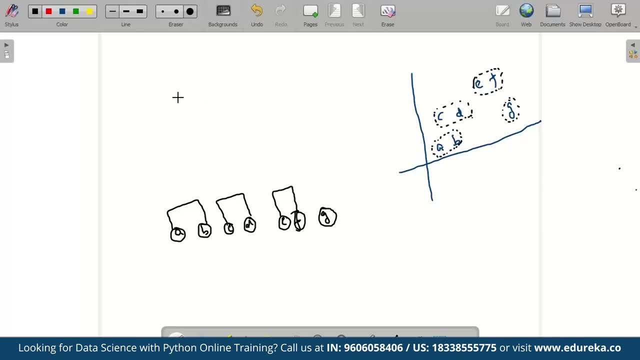 ungrouped, which is not being grouped into any of the cluster. so now clustering: I said that it is. it continues until a single cluster is left. so now I would have to have another level of clustering. that means that e, f, g- since g is very close to e f, I will cluster it in one single cluster. okay, and 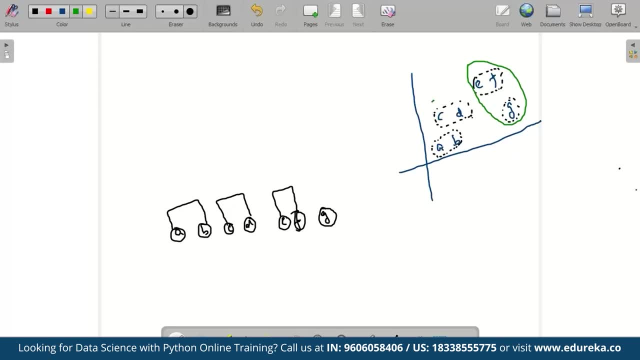 since I can see that both these a, b and c d pairs, these clusters are again together. let me just cross this line and I would make one single cluster of these four points right. so what I do is, since these two are connected, I connect them with the. 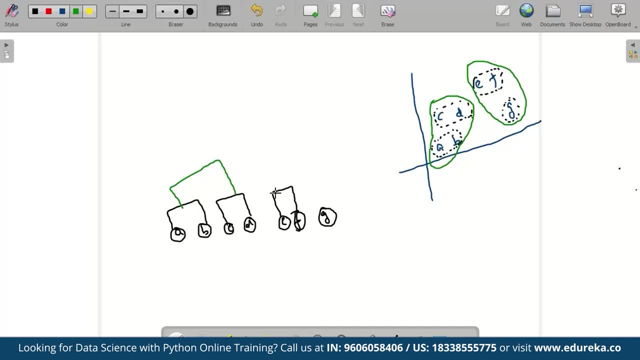 help of this line figure, that is restructured endogram, and this g, e and f. they are connected. somehow. I connect them all. right now. what happens is that I have got two big clusters and clustering continues until a single cluster is obtained. so in the end I will have to cluster. 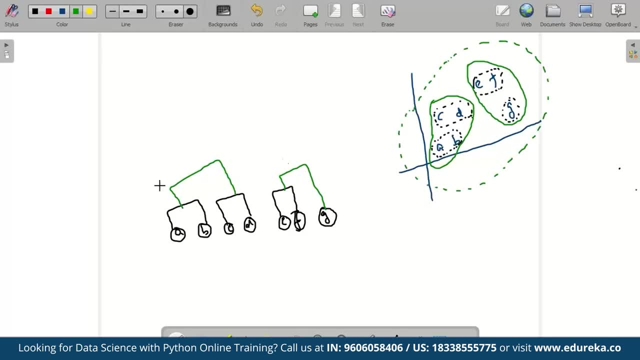 everything into a single cluster, and this is how I do that and to join it, I will again join this entire graph. so this is when it follows a bottom to up approach. this is called as agglomerative, hierarchical clustering. okay, so now we will go and see an example of 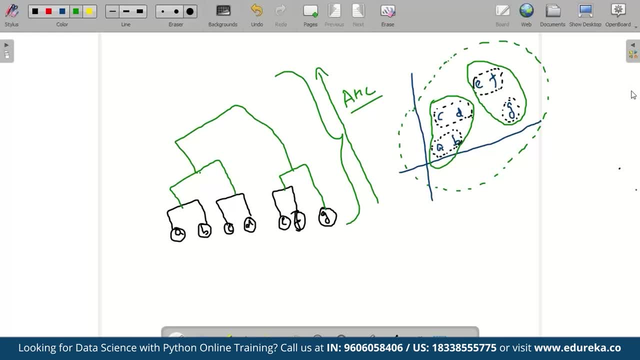 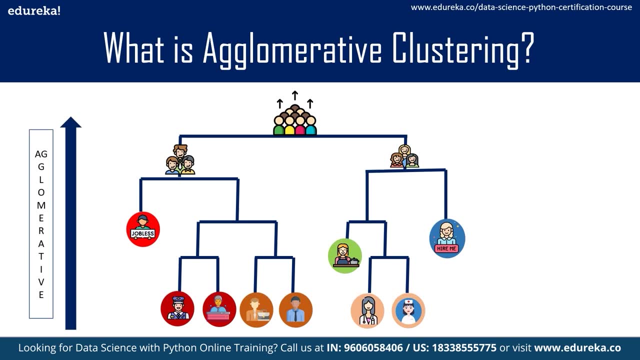 this hierarchical agglomerative clustering right, okay, so let us understand what is agglomerative clustering with this example. now we see that here the clustering takes place from bottom to up, and we have taken an example of population wherein we go on clustering until we get population. so here from 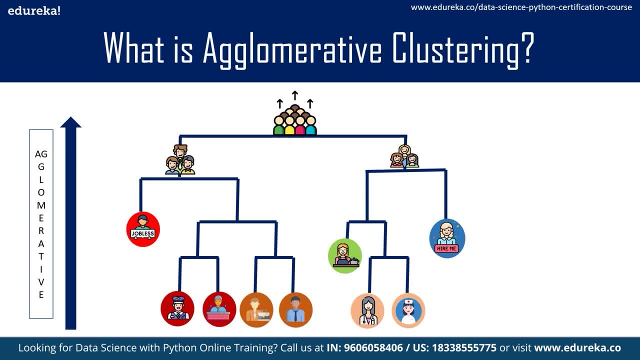 the bottom, the individual professions are being plotted and we see that let's, let's take for a convenience the left hand side and on the left hand side the red dots. as you see, this is individual profession in public sector and on the another side, which we see in the brown circles, is the 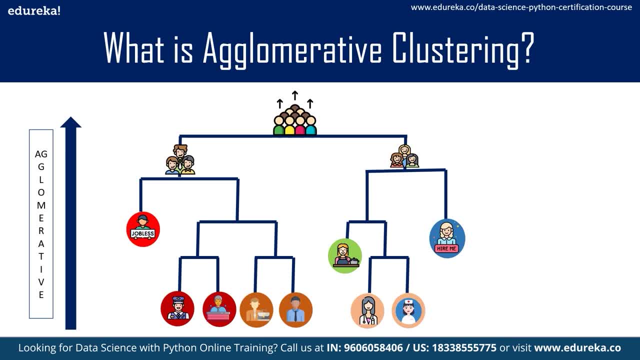 private sector, employment. so somehow there's similarity between private sector, so they are being clustered as one single cluster and the private sector as a another cluster. these again are being clustered into one single cluster and that is employment cluster, whereas on the another side we can see another cluster which is different and that is unemployed section of cluster of people. now they 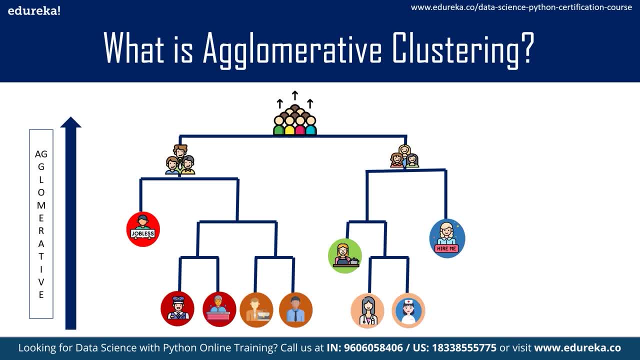 again share one similarity, and that is that they all belong to a single gender, that is male. so everything is being clustered into one single cluster, that is male. and then again male and female are being clustered together to form one single cluster, that is population. similarly, we also 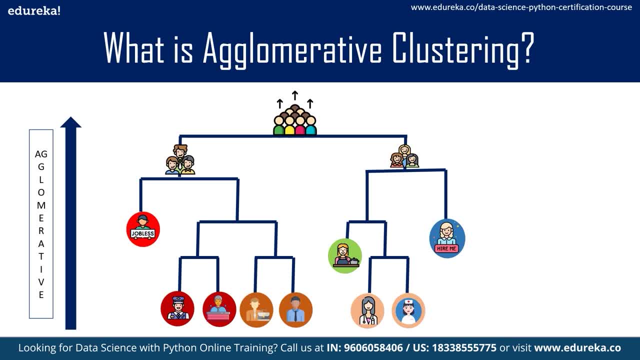 divide. on the right hand side, the individual professions of women clubbed into private and public sector, and then again we have separate clusters of employed and unemployed women and they have been grouped into one single cluster. that is woman. again, we merge the two big clusters into one single cluster, that is population. so this is how the clustering is taking place. the levels are. 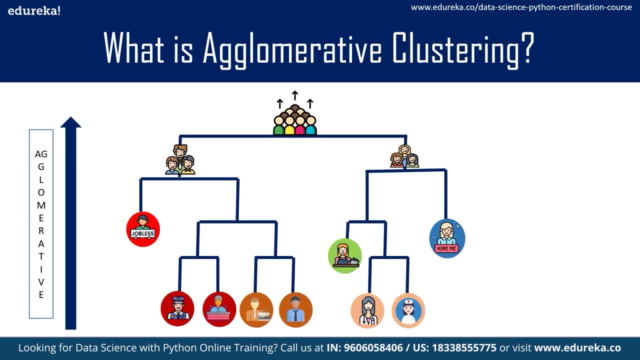 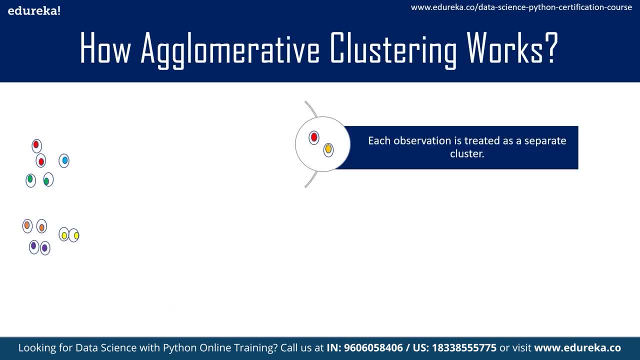 been increasing from bottom to up. So when we are using this bottom-up approach, this is agglomerative clustering. Okay, I think things are very clear now. So now let's move on to how does this agglomerative clustering work, and we will take this example as a reference. So now what? 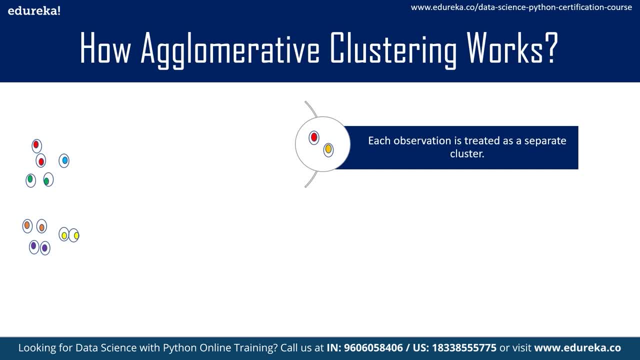 happens here is that each observation is treated as a separate cluster, which means that each individual profession was being treated as a separate cluster. and then these, the two clusters that were closest, they were identified and merged. So the public sector, which was closest, it was merged, and so on. Now, moving on further, the clustering continues and then again the clusters. 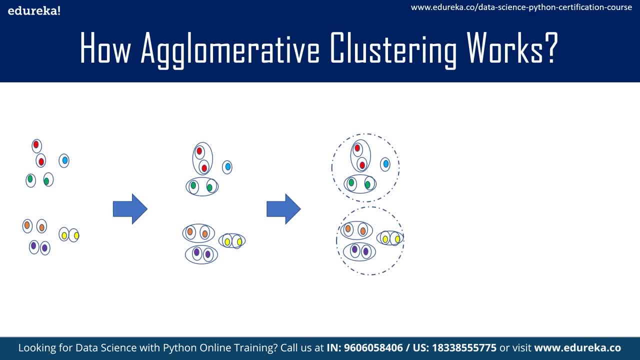 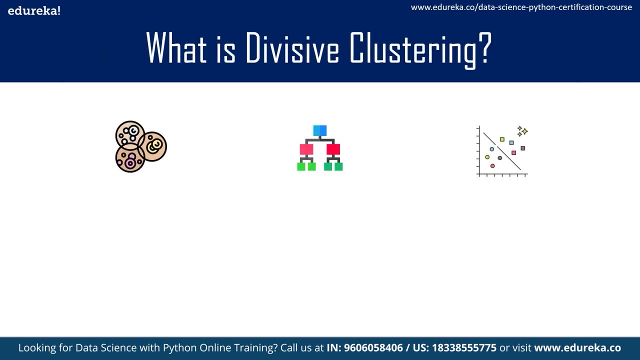 were being formed. when we see that employed and unemployed cluster, they were different and we go on clustering until we obtain a single cluster and that was population right. Okay, so now this was about agglomerative. and now moving on forward to what is divisive Clustering. now, in divisive clustering, this is also known as Diana, and this is divisive analysis. 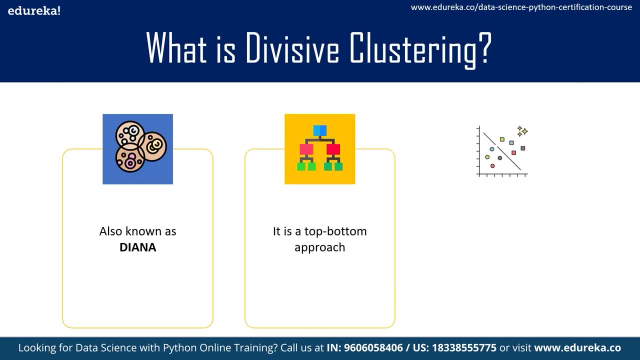 clustering algorithm, and this follows a top-to-bottom approach. This is just the opposite of agglomerative hierarchical clustering, and clustering continues until small groups of similar clusters are obtained here. This means that all the data points they belong to first one cluster and then the clusters they are formed as we move down the hierarchy. Now, having said this, let us understand. 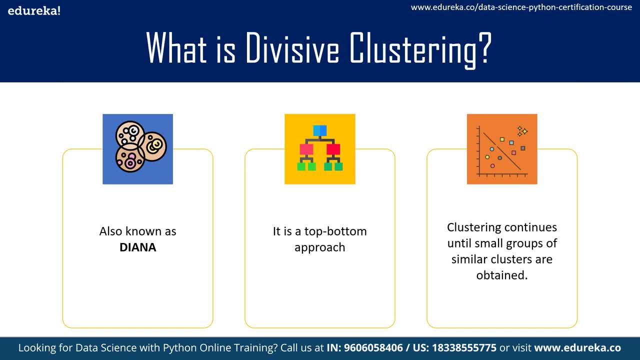 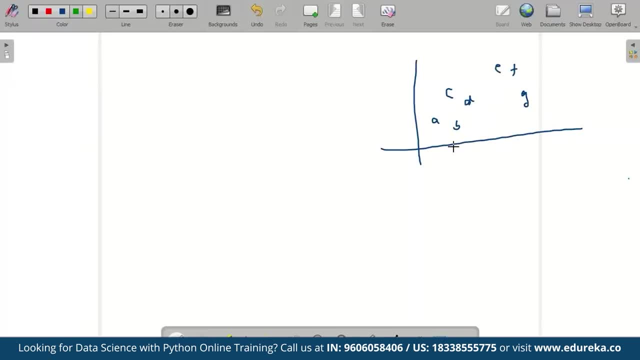 what exactly Is divisive clustering? and we will take an example and let's understand it by drawing first, and then we'll go on to understanding with the help of an example. So now let us understand how divisive clustering actually work. So now we've got, suppose, these data points scattered and let us now cluster. 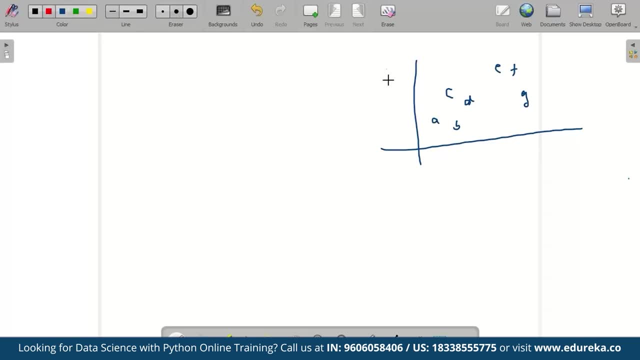 them. So for divisive clustering, what happens is that we start from one single cluster and we just cluster them into one single whole right, and then we will start clustering them. So what we're going to do is we will form another cluster based on the similarity, or you can say the: 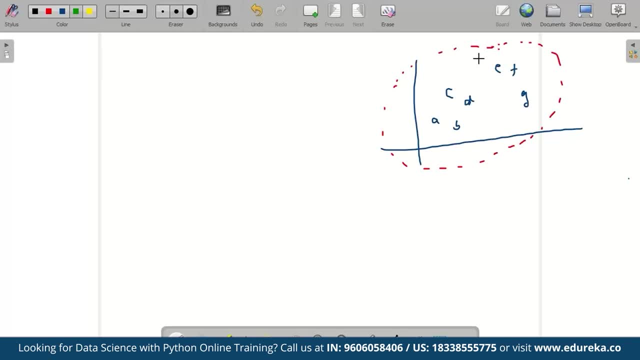 distance between EFG cluster. We see that these are near. so what I do is I form one single cluster of EFG and I see that these share some you know- distance. They are similar and they have shared the same distance and nearby, so I cluster them into one single whole. Ok, now I will go on dividing or 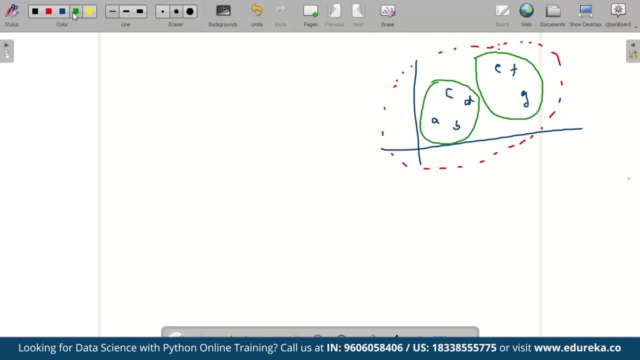 clustering until I get single unit of cluster. So I would go again further and let me take a different color. So what I do is I will cluster A and B into one single cluster and C and D again into similar cluster based on certain distance and which we 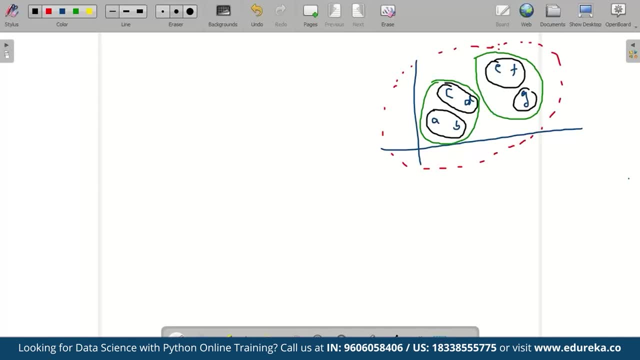 will study further And again we will cluster these clusters based on that: E and F are very near to each other, C and D are near to each other, and so on. Now the clustering is not yet complete because I have not got individual clusters, So what I do is I will cluster A and B into single. 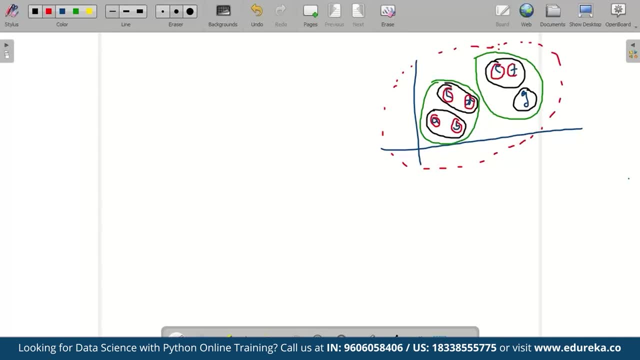 cluster again, and this would complete my divisive clustering, starting from one single cluster to boiling it down to simple small clusters, right? So if I want to just write it down into A, B, C, D, some kind of a diagram, So what I do is like similar figure I have, suppose I start from A. 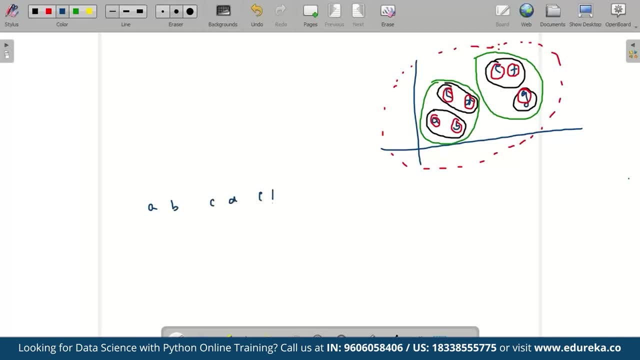 and B and C and D. So what I do is like similar figure I have, suppose I start from A and B and B and C and D. this is just same like agglomerative, but this, just the approach is different: A and B, and C and D. but what? 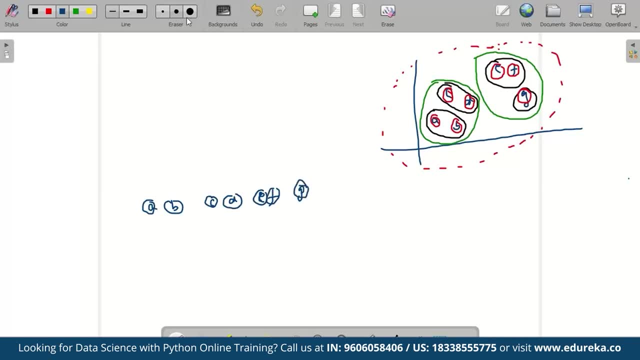 happens here is that when I'm moving a form forward from above. so I have all my data points here- A, B, C, D, E, F, G- and now I am moving on forward to dividing them into different clusters, which is suppose A, B, C, D, E, F, G. 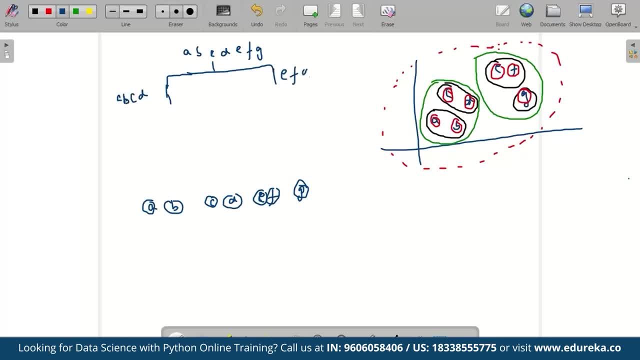 CD. here and here we have EFG, and then I will go on further and make for the cluster. for that I will go on. this is G- I know this is separate- and here this is E and F. so this is E and F, right, and this figure is nothing but a dendogram that I'm drawing. don't mind the lines here, just follow the. 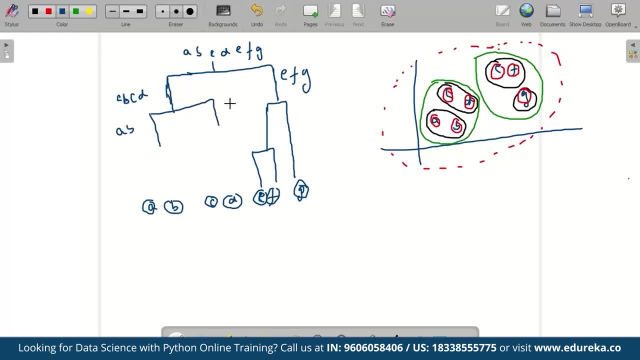 concept. and here I have here A, B and CD cluster and this has been divided into A and B and this is divided into C and D. right, so this is how the clustering takes place: dividing a single cluster, separating it down into separate clusters, and when I'm following a top to bottom approach, 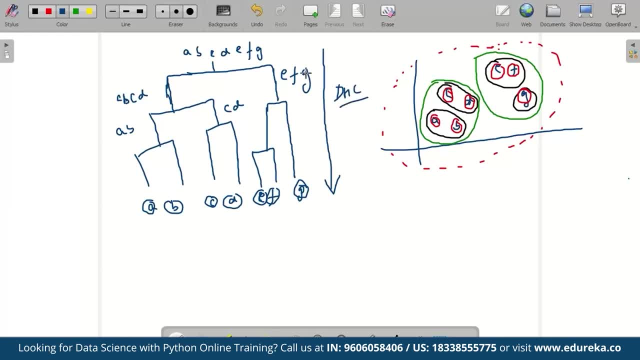 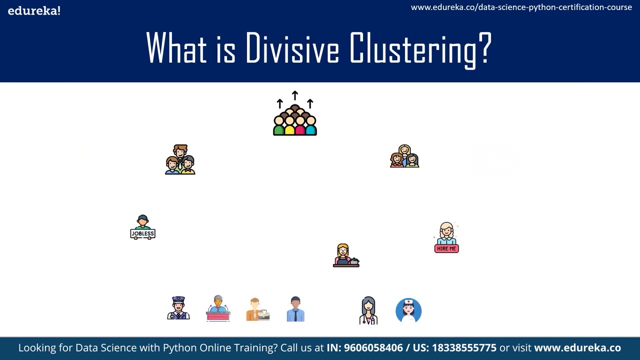 this is known as divisive hierarchical clustering. now let us understand this with the help of an example, and and make things more clear. this was just a rough, a vague idea about how this clustering is and how our dendograms form. so now coming to the same example of divisive clustering, and here the clustering takes place. 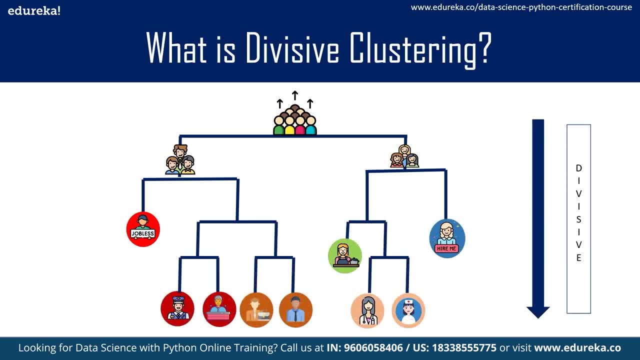 from top and we have the population, which we divided into male and female clusters, and moving on for further. the male cluster is divided into employed males and unemployed clusters- male. and again the cluster is further divided into the private sector employed males and the public sector employees- male. similarly, we can replicate: 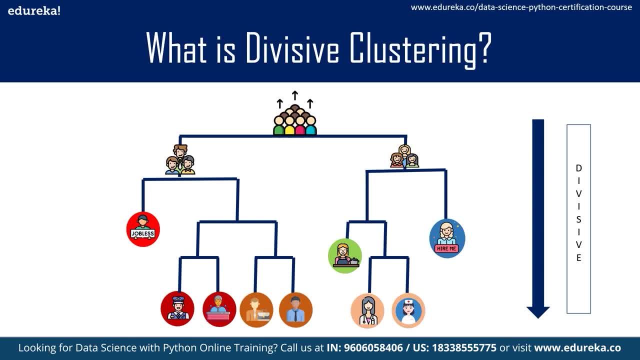 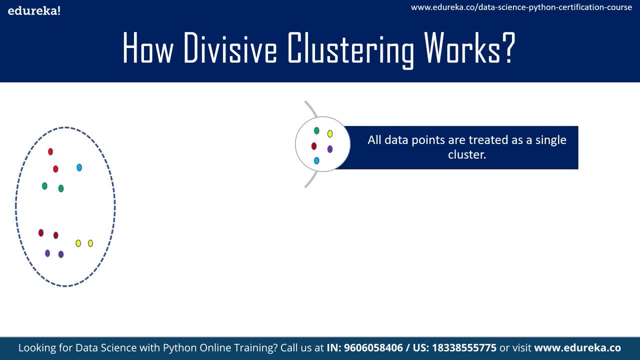 this with the female clusters also. so this is how divisive clustering approach approaches from top to bottom clusters, and this is divisive clustering. now let's move on further to how does this divisive clustering work? so all the data points are treated as single clusters and then the cluster is partitioned into two least similar cluster, and then again the clustering takes. 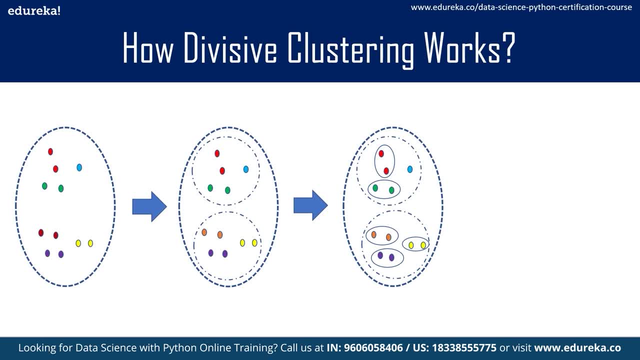 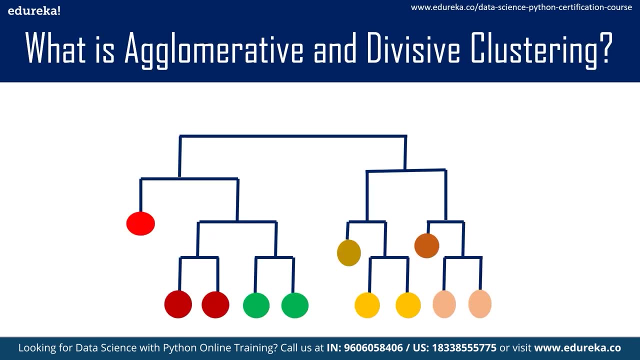 place based on certain similarity between the clusters, and then further when we, until we, get a single individual cluster within a cluster, and this is how divisive clustering will take place till the end. now let us understand what is a glomerative and divisive clustering just in a 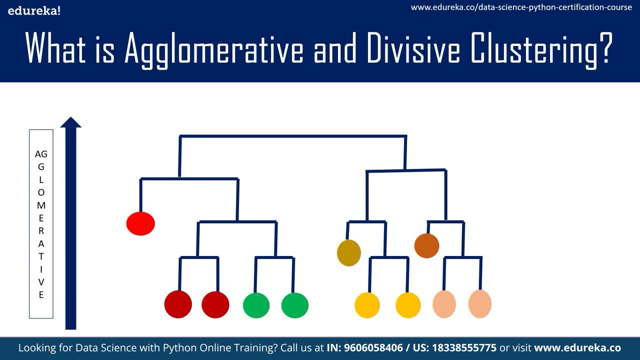 nutshell. so when you're moving from bottom to up, it is a glomerative, and when you're moving from top to bottom, that is divisive. alright, and this representation is called dendogram, which we have seen and we have plotted, and we have seen it in the example too. okay, so now moving on forward, let us understand. 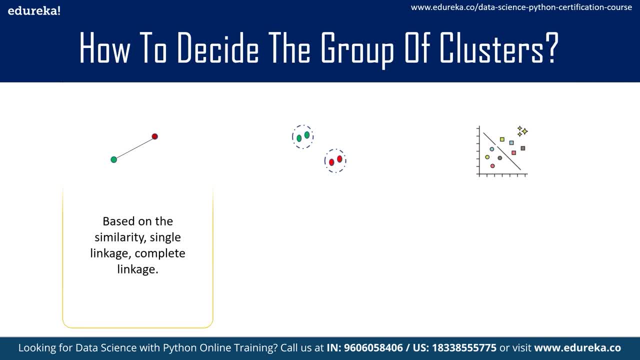 how to decide the group of clusters. so it is done based on some similarity between the data points that we have seen, and the similarity could be single linkage, complete linkage, median linkage, centroid linkage, and which we will discuss it also, and it is now similarity. another thing is: 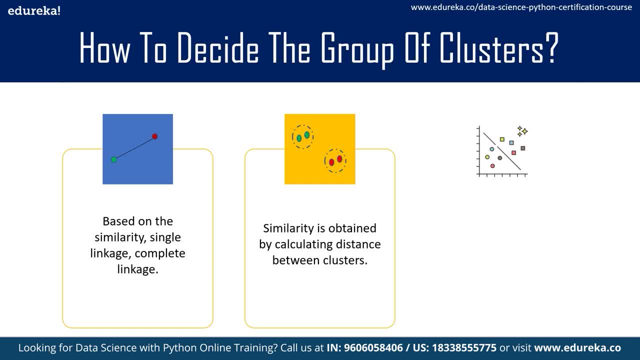 that the similarity. it is obtained by calculating the distance between the clusters and the. generally the distance matrices used are Euclidean distance, Manhattan correlation distance. even Minkowski distance is used. so now, generally the Euclidean distance is used to figure out the distance between the data points, but the choice of a distance matrix again depends upon the 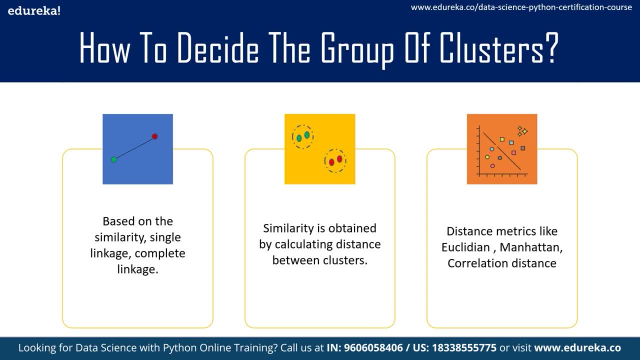 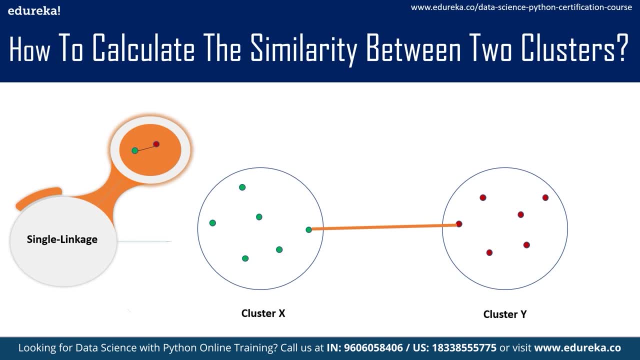 data set under study right like for example, in gene expression correlation, distance is often used. so now, moving on further, how to calculate the similarity between two clusters? now, here we have got two clusters like X and Y, and to find the similarity between two clusters, single linkage technique is used here. what happens is that the distance between two most similar parts of the 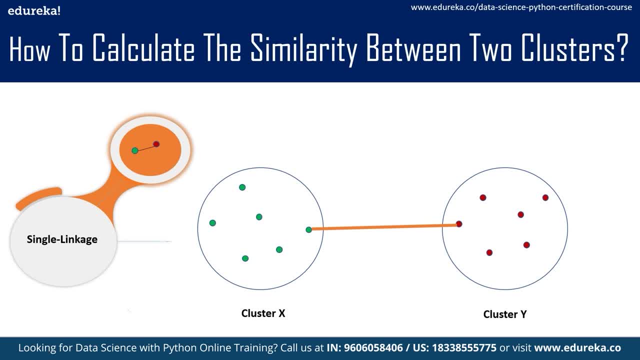 cluster is being taken, the distance is mapped, and this is how clustering takes place. another way is complete linkage in complete linkage again, what we take here is that we take two least similar bits of cluster, that is the farthest point in the cluster. that distance will be taken, and then 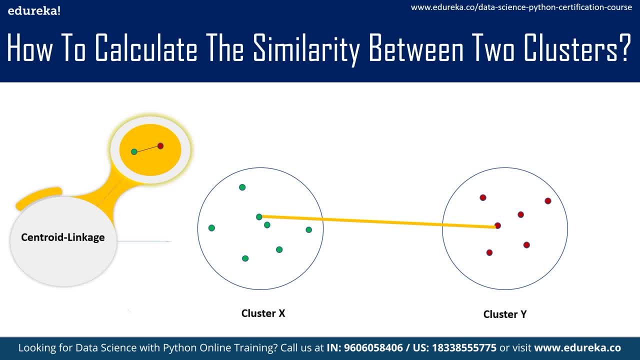 the clustering is done. another way to cluster the data or to form clusters to find the similarity between cluster is centroid linkage. now what happens is that the distance between centroids of the two cluster has been taken. there are other methods also, like mean or average linkage, where the center of the cluster is taken. and now remember, here centroid of the cluster is taken, which is 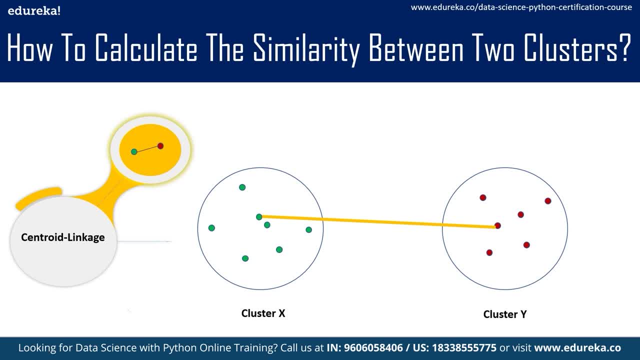 different from mean or average right. and there is yet another way of linkage criteria, like words of the square of euclidean, distance is minimized, all right. so, depending upon the data set we will choose, or the hierarchical clustering will choose which method, which distance, which matrix to be. 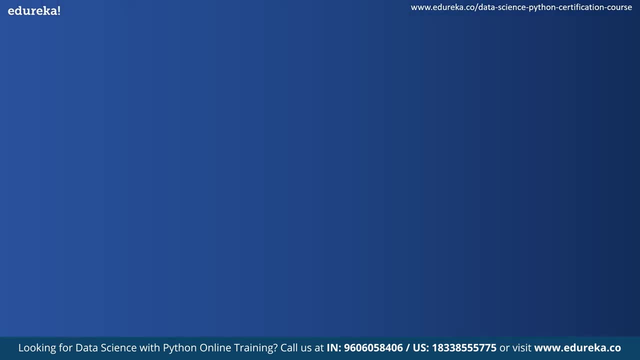 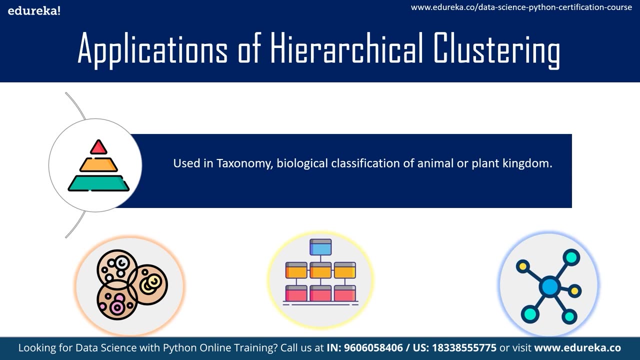 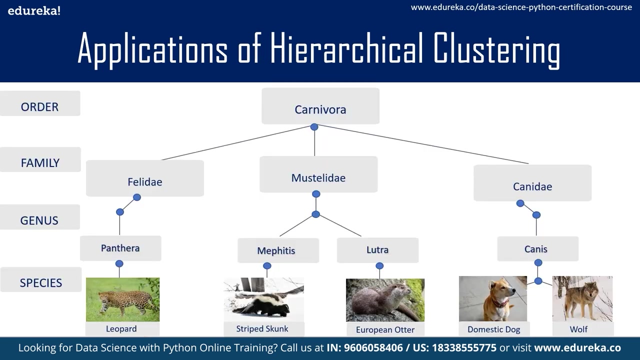 applied right. okay, now, moving on further to some of the applications of hierarchical clustering. hierarchical clustering, now this is used in taxonomy, which is the biological classification of animals and plants kingdom. so let us understand this with the help of an example. now, this is the example which we are going to look at in the next video. so let us understand this with the help of an example. now, this is the example which 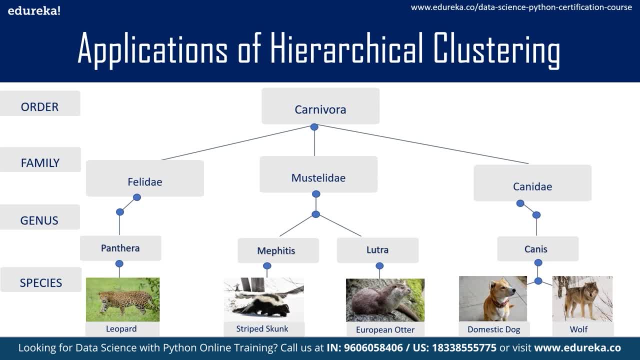 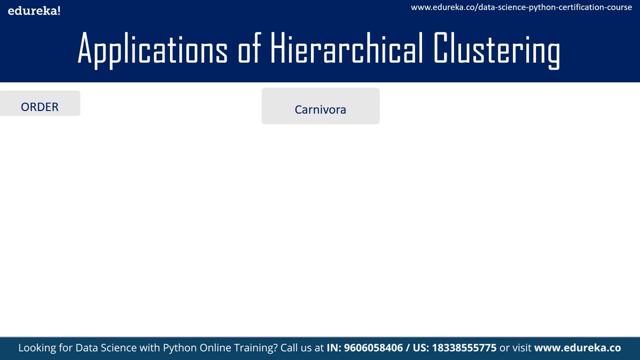 we will be understanding and how the classification takes place. so now we start with the first order. that is the first level of cluster, that is carnivora, and it falls into order. right another, it has been divided into the family of felidae, mustelidae and canadae. right now, these are some. 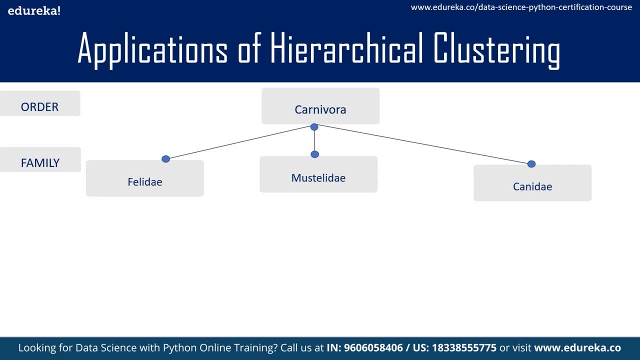 scientific names. but when we reach the end we will understand what this really means. so don't worry if you're not from like scientific or biological names, friendly, never mind. now, another level is genus. so these, this family is then further divided into the genes of a species which is panthera mephitis, luthra, canis, and again, this has been further. 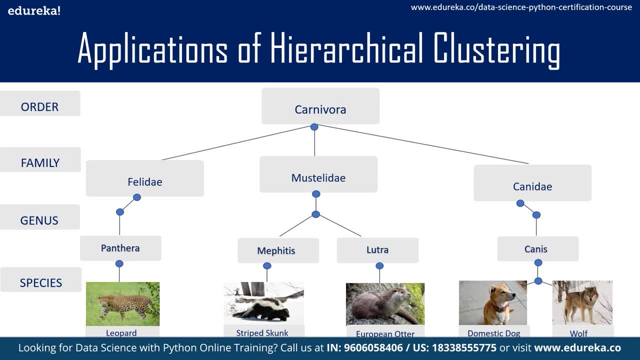 divided into species. so until we get individual clusters of these species, we will keep on clustering them into various levels. so the species are: leopard- here we have got striped stung european otter, and in canis we have got domestic dog and wolf. right, so domestic dog and wolf. 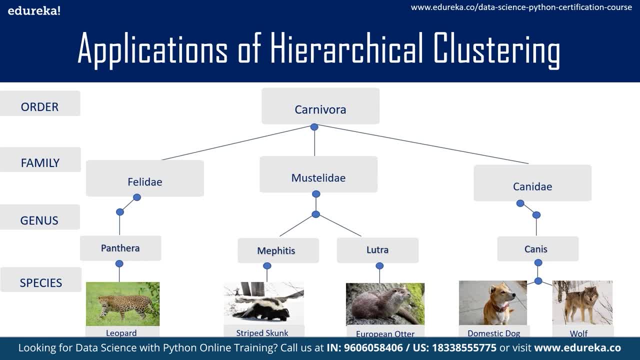 share some similarity. that's why they have been clubbed into the same species, and then they have been clustered into canis, because they are carnivores, and then, but their family is canidae, which is different from felidae and mustelidae and but just forming the one single cluster, that is. 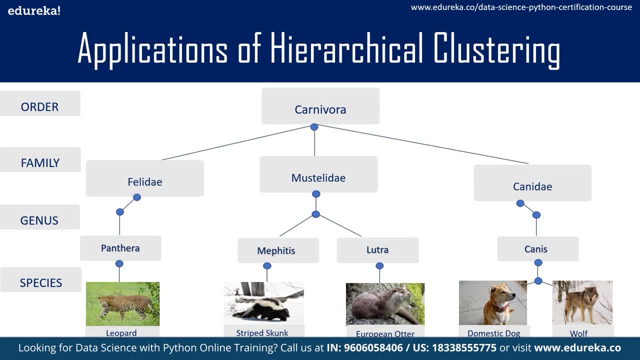 carnivora, right. but these individual species, they have certain dissimilarities between them, but they fall under the same family in the same order. right, the same order, not the family. okay, so this is how the application of hierarchical clustering finds its usage in taxonomy and biological classification of animal and plants. now moving on forward to other 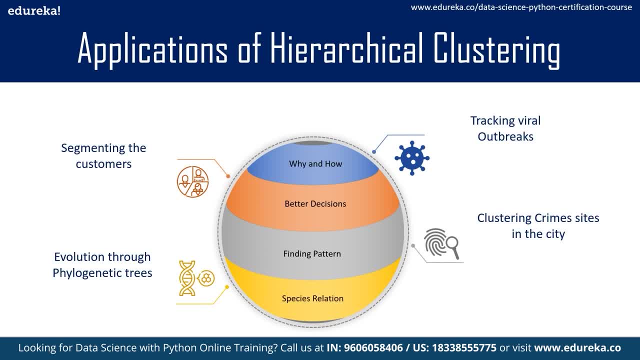 applications of hierarchical clustering is tracking the outbreak. so hierarchical clustering is used to track the virus and their sources and this is really very useful for scientists because this gives understanding of the virus source, the origin of the outbreak, like why and how the outbreak began, and potentially they can save life. 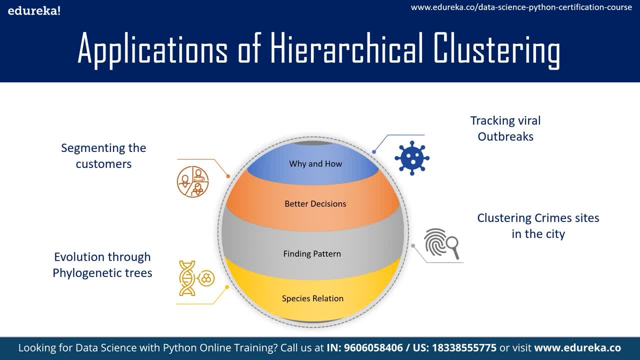 and then another important application is clustering crimes in the city so the lawmaking agencies and the police involved can really understand the trends and the patterns in the data and classify the crimes accordingly and take strict actions as per the crime. so need for more strict laws and clusters which are having high number of like murders or assaults or rape cases. 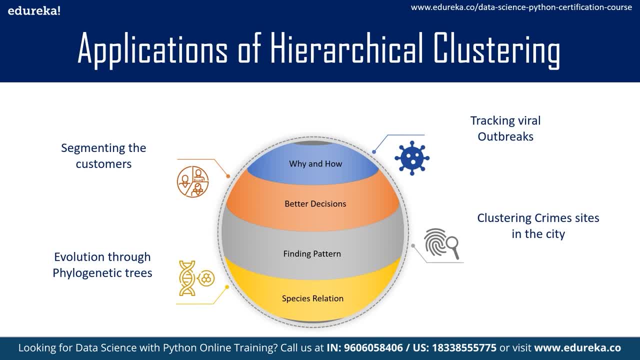 and this clustering really helps in understanding the trend, the pattern in the data and accordingly, then data-driven decisions and actions can be taken. yet another important hierarchical clustering application is evolution through phylogenetic trees. now, this means that to find how different of species relate to each other. now for this, what we take. 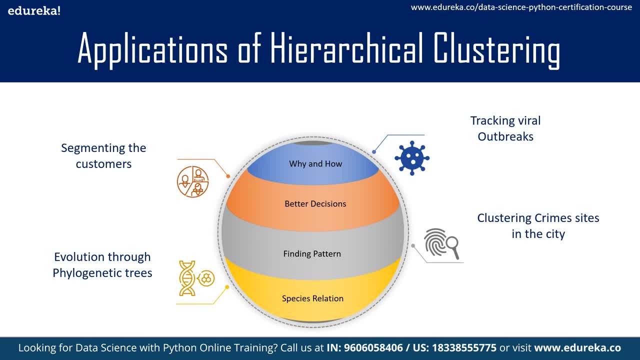 dna sequencing and hierarchical clustering. they have been used together- and the dna sequence of the species. they are generated and similarity in the dna is found by calculating the distance between the sequences. based on this, phylogenetic tree is constructed and this really helps in classifying or placing the new discovered species into the gene chart or into the the family. 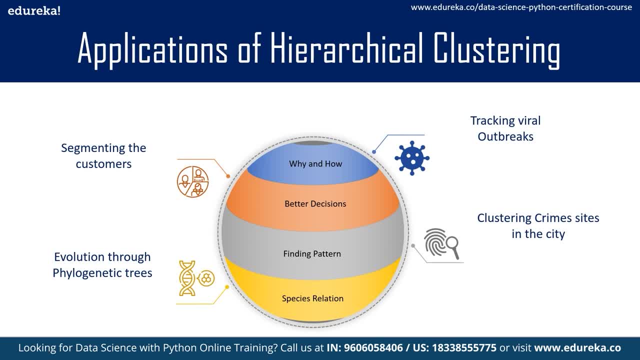 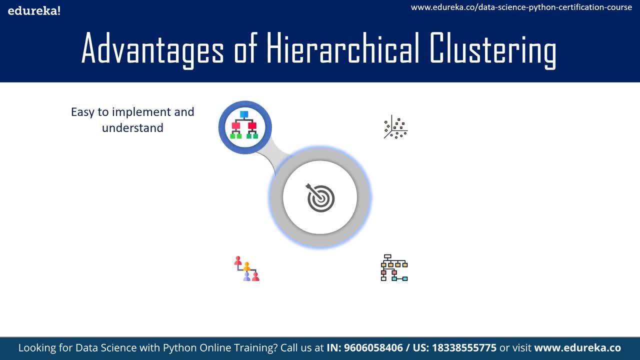 or the order of species, right. so hierarchical clustering is really useful for that. now moving on forward to the advantages of hierarchical clustering is that it is easy to understand and implement and gives better results in certain cases too. here we do not need any pattern information about the number of clusters, unlike in k-means. 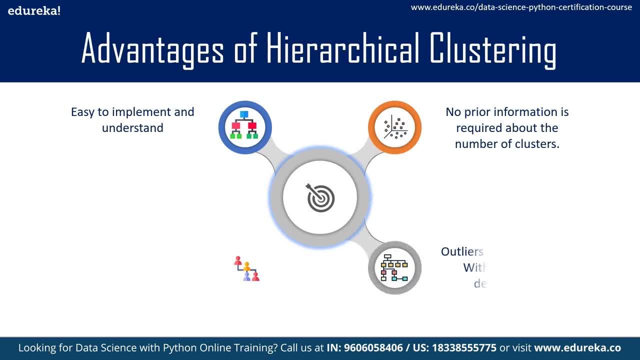 where clusters have to be pre-assigned. the another advantage is that the outliers can be detected with the help of dendograms, and it also gives insight into the data structure. so another advantage is that hierarchical clustering is more deterministic and more predictable, whereas k-means with random initialization can produce different results when we run the. 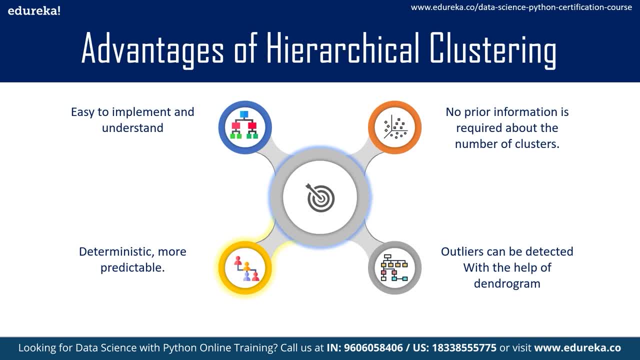 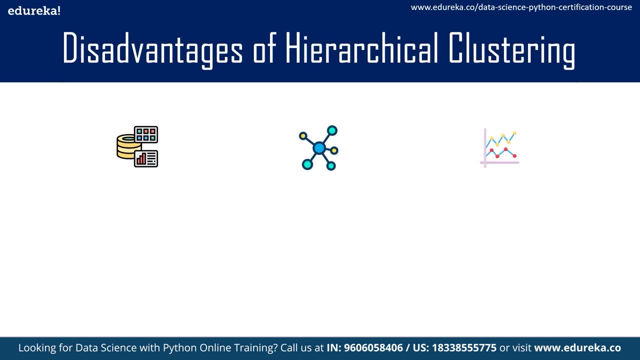 same data multiple times. so hierarchical clustering will give you the same results whenever you run it multiple times, so this is more predictable. now moving on forward to the disadvantages of hierarchical clustering is that it is not suitable for large data sets because of large space and time complexities. time complexity of at least o? n squared log n is required. 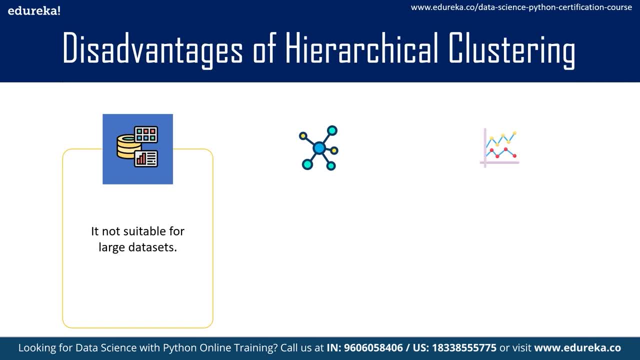 where n is the number of data points. so you can- you can really imagine that how much space and time complexities are involved with hierarchical clustering. now, another disadvantage is that it is difficult in handling different sized clusters and convex shape. also, at times it is really difficult to identify the correct number of clusters.